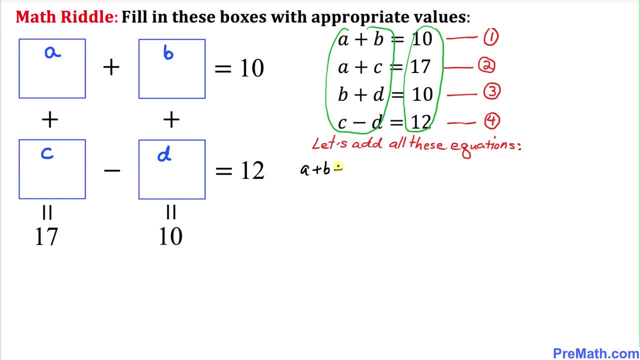 a plus b plus a plus c plus b plus d plus c minus d equals to: now let's add the right hand side numbers. those are 10 plus 17 plus 10 plus 12. all right, so our next step: we are going to combine the like terms, this a and a, that's going to become 2a. likewise b plus. 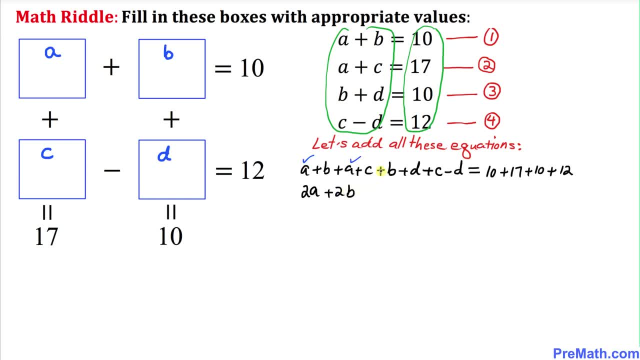 b is going to become 2b and c, two of them c, and we can see that this positive d and negative d, they cross out, they are gone. that is equal to when we add the right hand side number. that's going to give us 49 and we can see, on this right left hand side we can factor out two. this is going to become a. 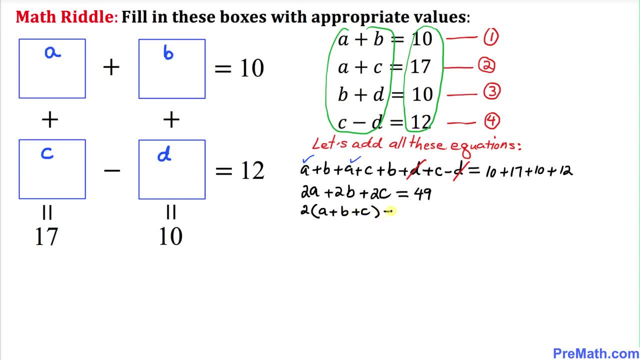 plus b plus c, equal to 49, and now i am going to divide both sides by 2.. so that means this 2 is gone. so that is going to give us a plus b plus c equal to when we divide 49. divided by 2, that is going to give us 24.5 and therefore i have nicely wrote down a plus b plus c, equal to when we divide. 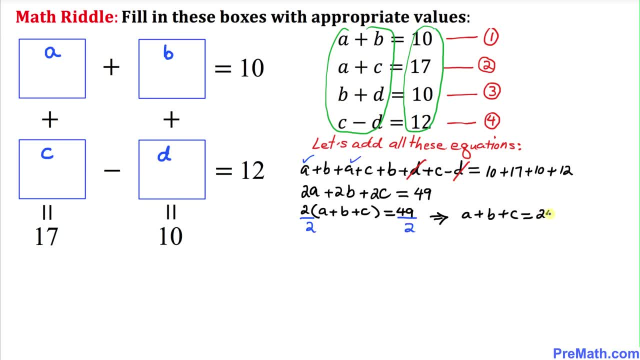 49 divided by 2, that is going to give us 24.5, and therefore i have nicely wrote down: a plus b plus c equals 9.. и discussion senses that fact that we six clearly haveimporte if we are getting eight times even f. i never think about this situation and therefore i have never. Но難為 Barbadi, is that presseti re guesht hat er. 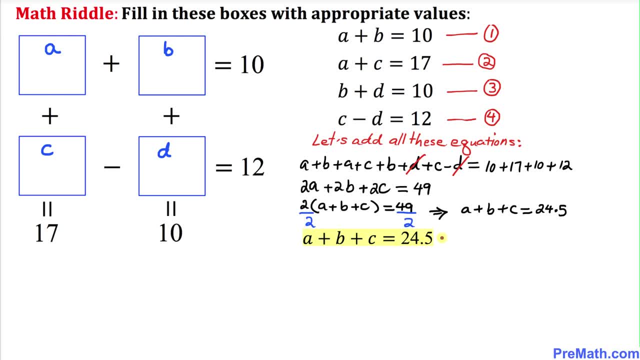 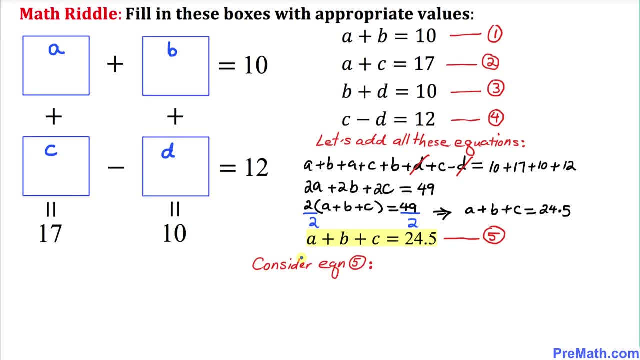 plus b plus c equals to 24.5. and i am going to call this equation as number five. and here's our next step. let's consider this equation number five, and here i wrote down: a plus b plus c equals to 24.5. and as we can see that a plus b by just looking at this equation number one, we can see: 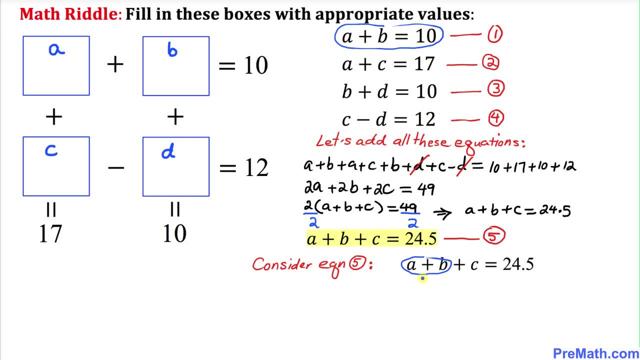 that a plus b is 10. i am going to replace this a plus b by 10, and then plus. this is going to become plus c equals to 24.5, isn't it? let's move this 10 on the other side, so c is going to be 24.5. 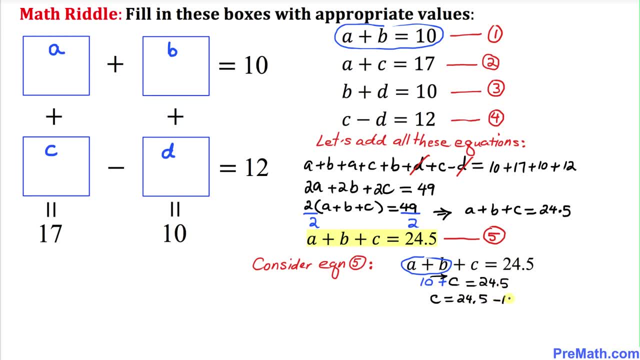 when we move, 10 on the right hand side becomes negative 10. so that's the equation number five. and here's our next step. let's consider this equation number. that means c is going to give us 14.5. so thus our c value turns out to be 14.5, and i am going to write: 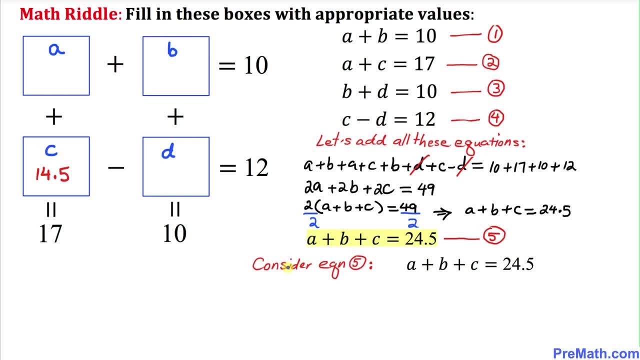 down in this box. and now let's go ahead and repeat the same process all over again. let's consider equation five once again, which is right up here. let me rearrange this one a little bit: a plus b, written as i can write, a plus c plus b equals to 24.5. it doesn't make any difference. and now let's 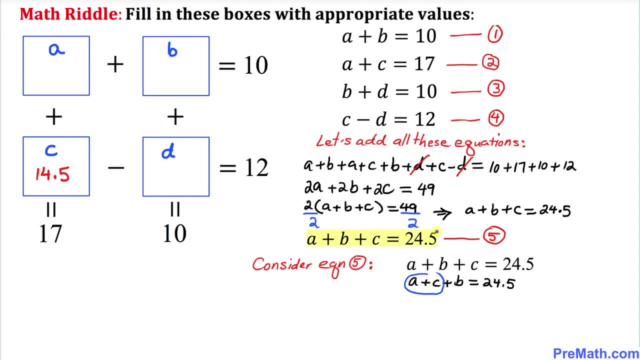 look at a plus c part and by just looking at equation number two, we know that a plus c is 17. i am going to replace a plus c by 17, and i am going to replace a plus c by 17, and i am going to. 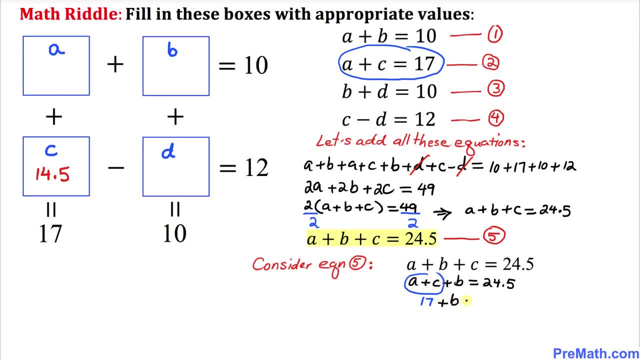 replace a plus c by 17 and then plus b equals to 24.5. let's move this 17 on the right hand side, so b is going to be equal to 24.5 minus 17. that is going to give us b equal to 7.5. 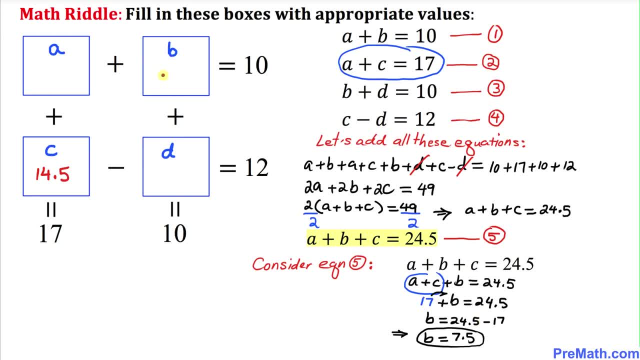 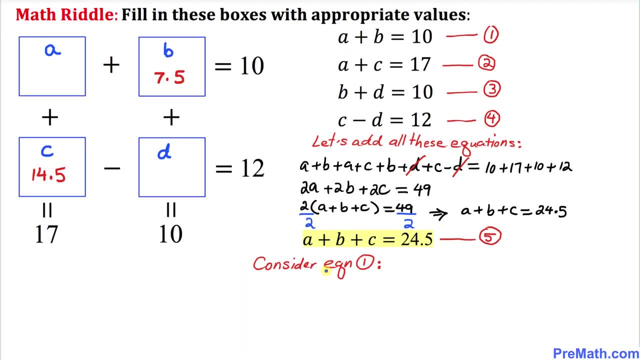 so that's our value. so thus our box b is going to have a value 7.5, and this time we are going to consider equation number one, which is right up here, and here i wrote down: a plus b equals to 10, and look at this b value b. we just figured out 7.5. let me just go ahead and replace b by.